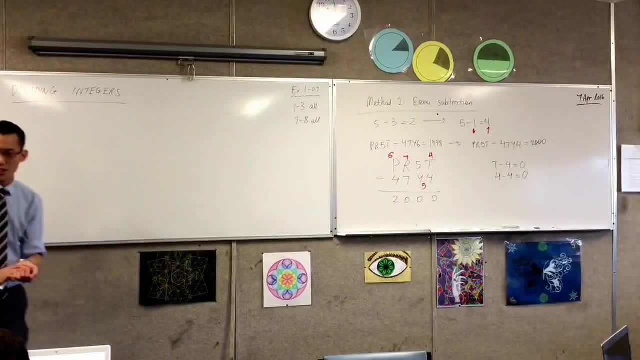 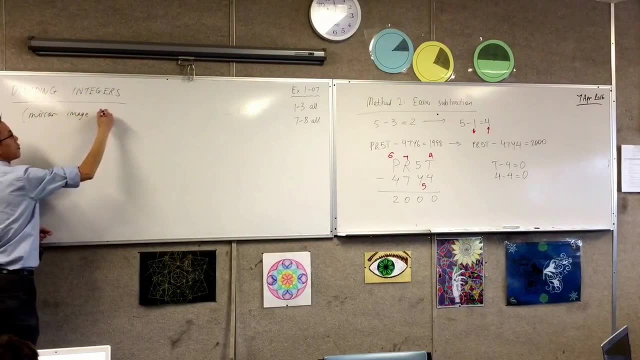 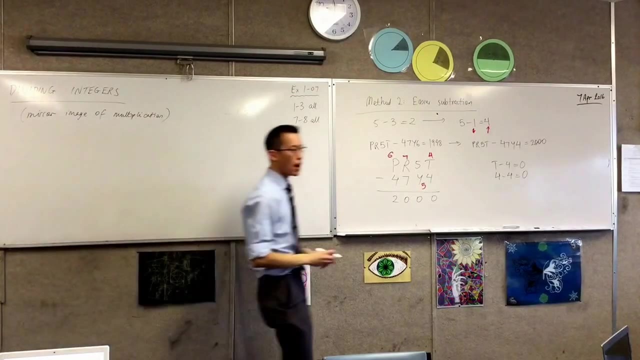 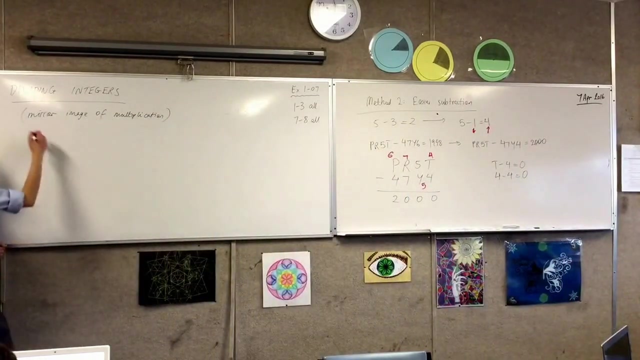 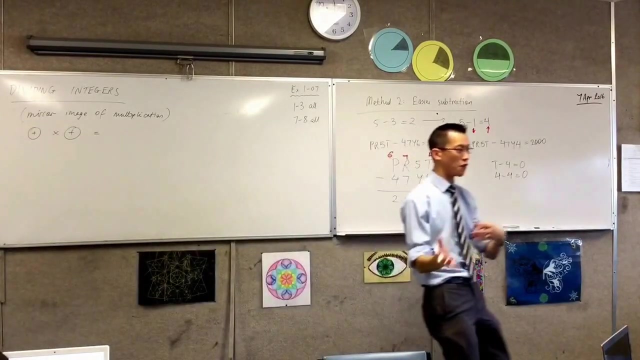 When we look at dividing integers. right, dividing integers is really a mirror image, and I'd like you to write this down. it's a mirror image of multiplication. So everything we knew about multiplication will apply when we think about division. For example, we know that when you multiply two positive numbers, positive times positive, what is the sign- positive or negative- of the result? the product, It's positive, right, Positive times positive. That's no surprise. 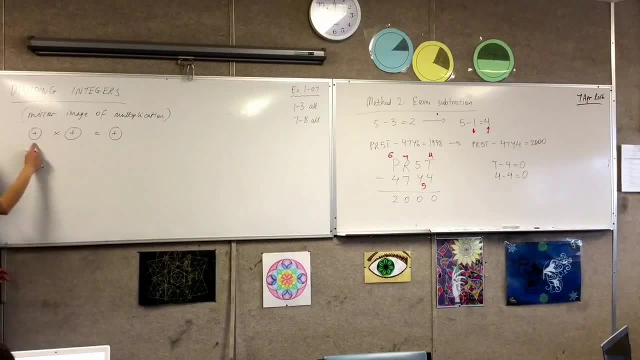 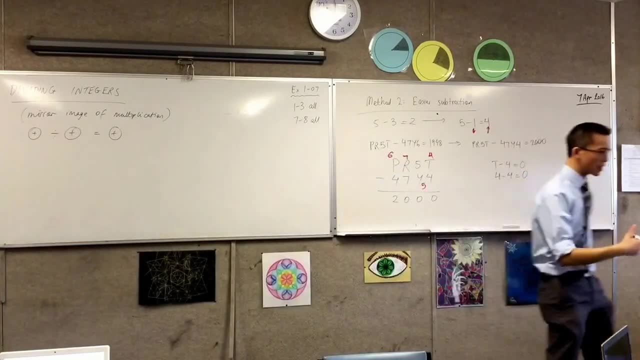 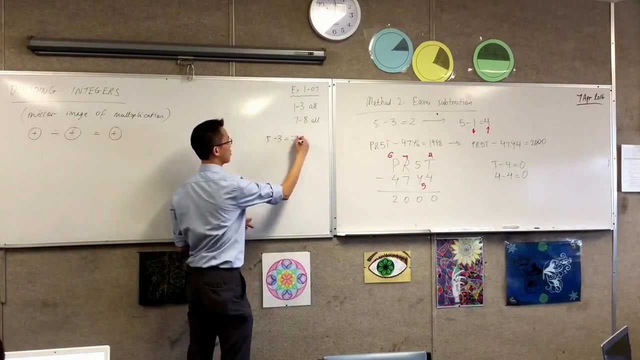 So, in exactly the same way, positive divided by positive will also be positive, right? Because multiplication and division are really just mirror images of each other, Just like before. you know how I said: oh, 5, take away 3 equals 2,, 2 plus 3 equals 5.. It's the same kind of relationship happening, okay. 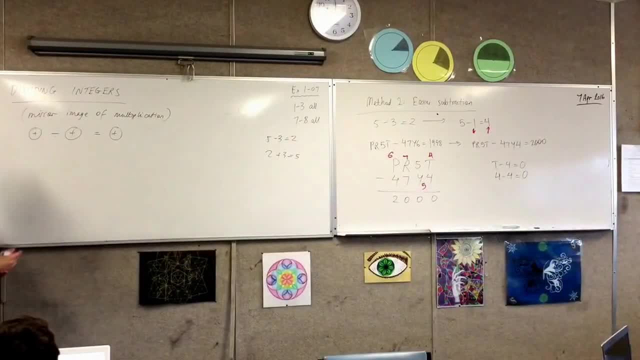 What were the other results we had before for multiplication? We had plus and minus. What happens when you multiply plus and minus? Yes, Sharon, You get negative. very good, So if you multiply them, and that's the result, when you divide them, that will also be the result. Make sense. 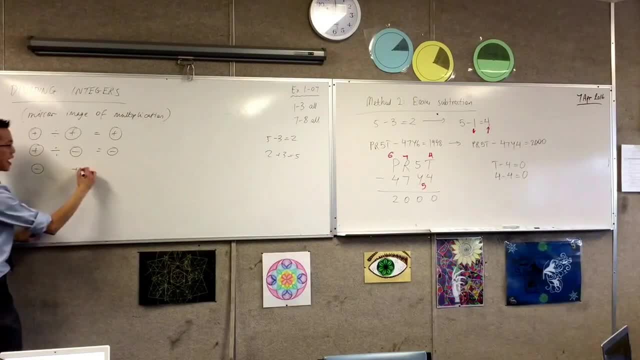 What if I switch the order? What if I have the negative first and the positive second? What happened when we multiplied those? When you multiply a negative times, a positive again- yeah, Rinesh, Negative, You get a negative right. It's still the same. And so, just like it is with multiplication, it's the same with division. 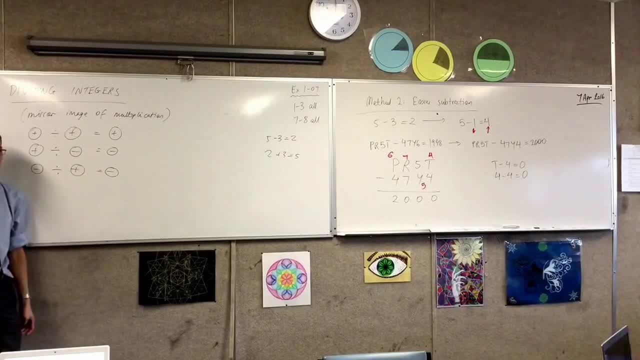 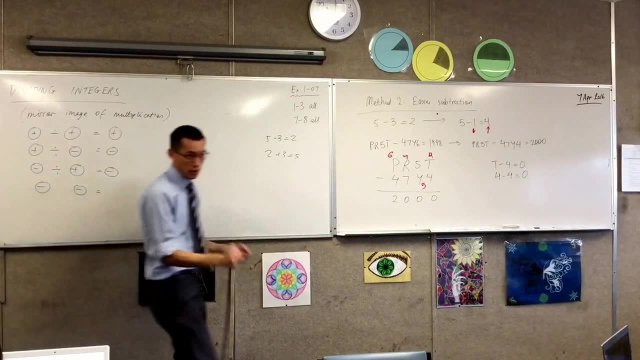 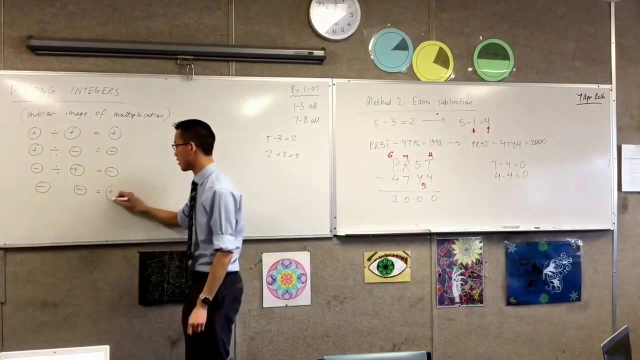 There was only one last combination that we had. when you got two different numbers right. What was the last combo? Yeah, Marley, Negative divided by negative. Very good, So negative and negative. So what we saw: when you multiply negatives, if you got both negative, you end up with a positive. and in exactly the same way, if you divide a negative by a negative, you also get a positive. 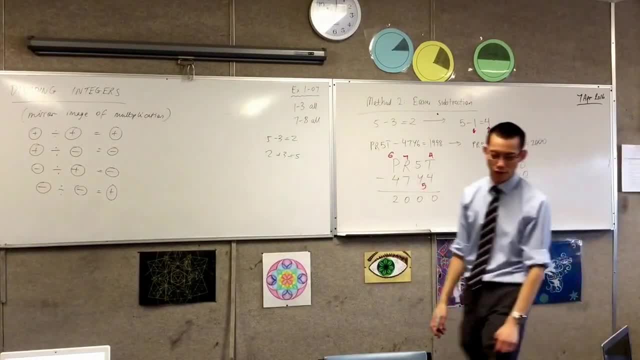 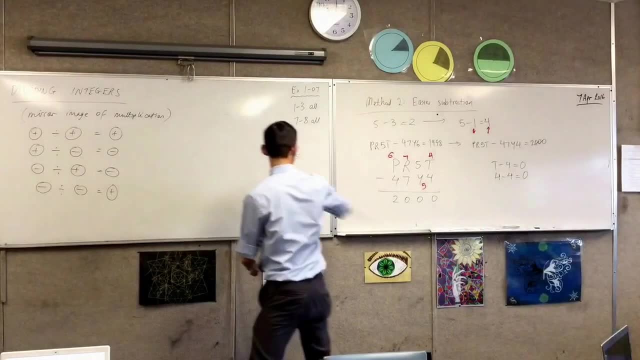 So this is not complicated, right? Let's have a look at a few brief examples. So you've got 107 there in front of you. Let's have a go at the first handful. So I'm going to start doing something for you. You're welcome. 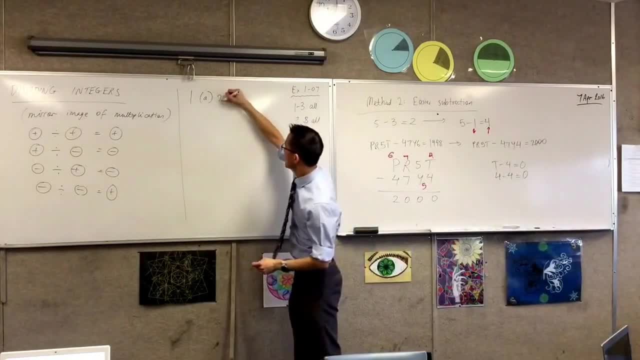 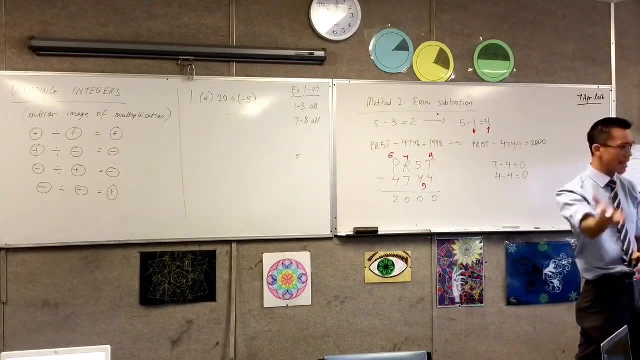 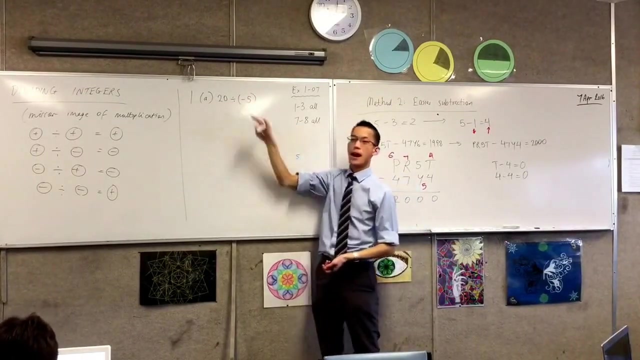 Okay, We have a look at this first question right: 20 divided by negative 5.. And please do get in the habit, like I've been saying before, about noticing that negative and minus are not the same thing. So I'm going to say 20 divided by negative 5, not 20 divided by minus 5.. It's not minusing for me. 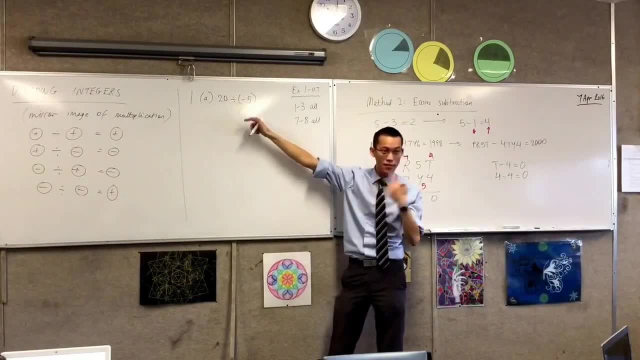 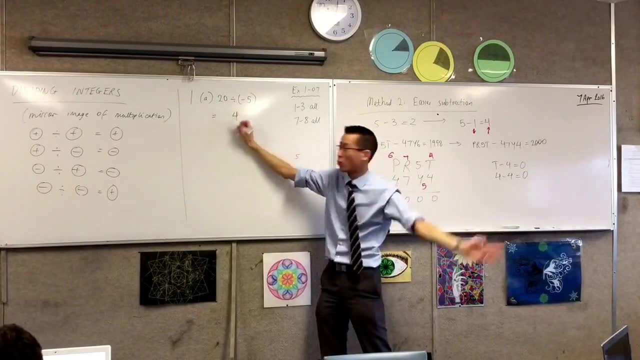 This is- let's think about the numbers first: 20 divided by 5.. 20 divided by 5,- you guys can do that- Negative 4.. Okay, so just the numbers. Negative 4, and I notice that there's a negative. One of them is negative, so I've got a negative 4 out the front. 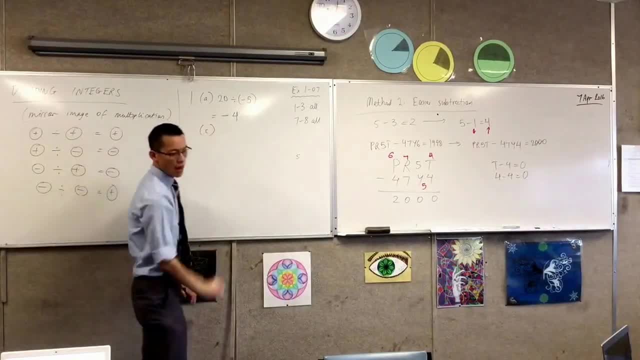 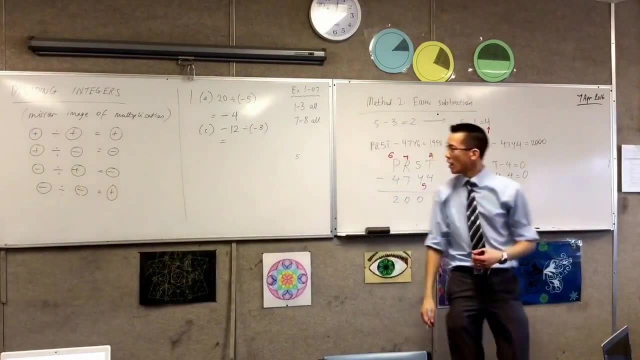 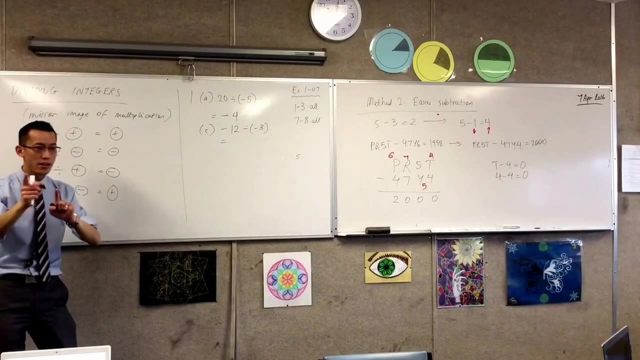 How about one, like let's skip over to C? I've got here negative 12 divided by negative 3. Okay, have a look at that one. What are you guys making of that Negative 4. Okay, now let's have a look. There's not one, but two negatives. right, Two negatives? 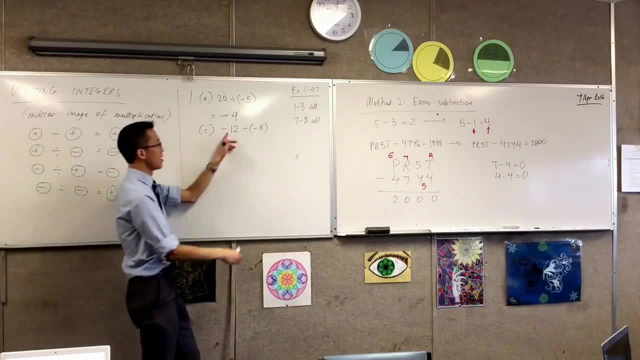 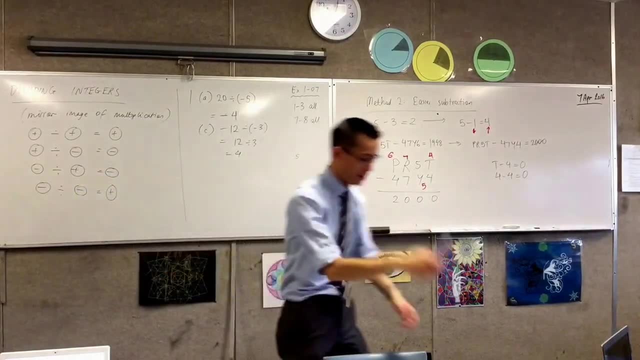 So that's this guy down here, right? So this is going to be just 20.. Negative 12 divided by 3, which is 4.. Okay, now, just underneath that, I want you to write something extra. Yes, Hannah. 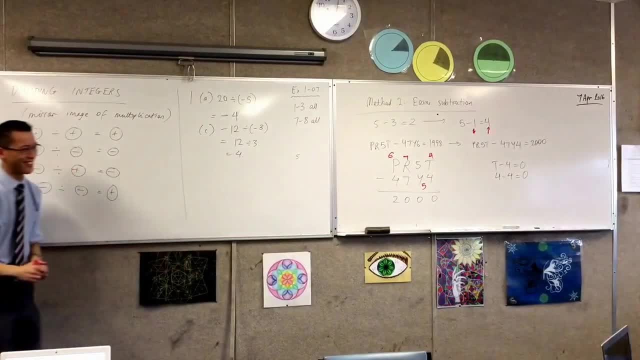 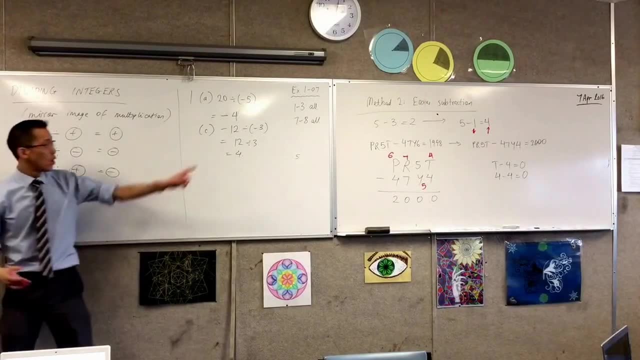 Can I get back my pen? I don't have a pen. Well, it's kind of my pen. It looks like a pen. Let's keep our belongings to ourselves, please. Yeah, Now let me try and help you see what's going on here and help you explain a little more, alright. 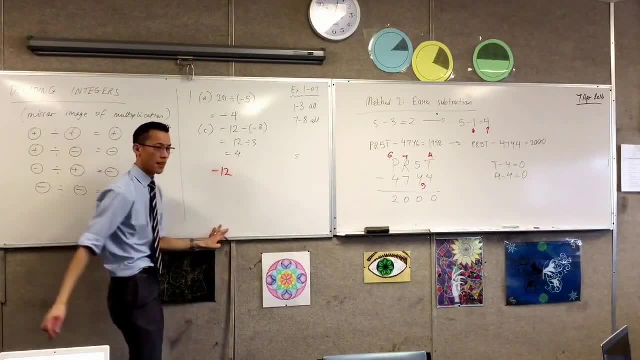 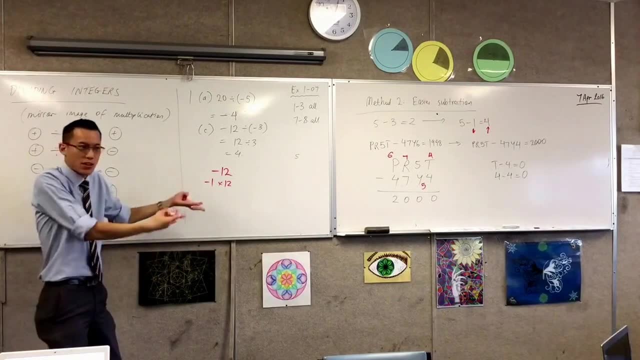 Negative, 12.. Negative, 12.. Right, I can write that as negative 1 times 12.. Do you agree with that? Like that's just how it is. I'm just having a negative sign out the front. So this is the same thing. 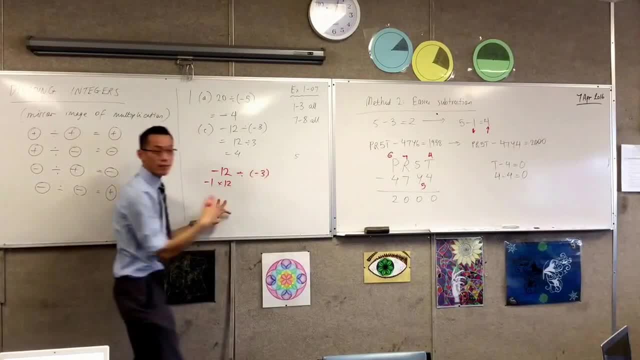 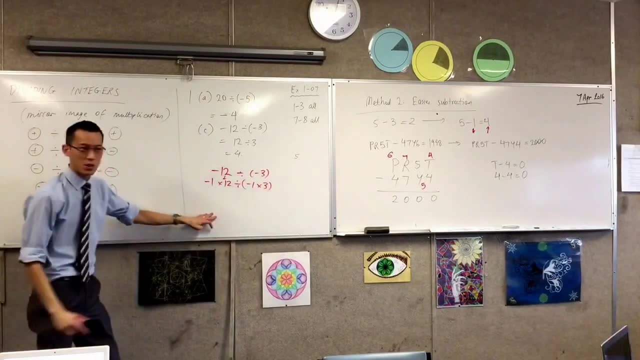 In the same way, negative 3, I can write that as negative 1 times 3.. Is that okay? Do you see what I've done? So here I've got one pair out of this number and another pair out of this number. 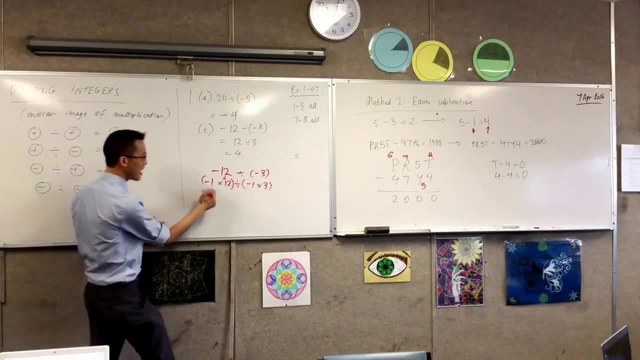 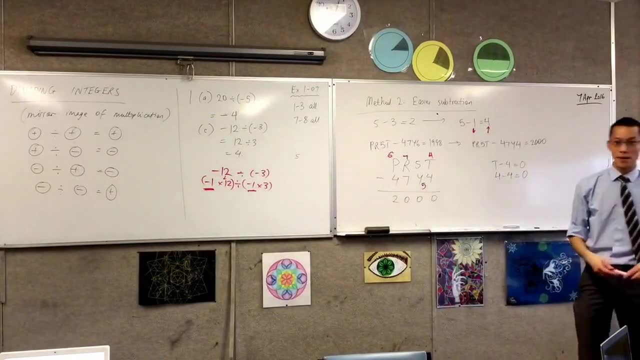 But remember, I can rearrange things here. right, I've got negative 1 and negative 1.. When you divide a number by itself, like 5 divided by 5, or 60 divided by 60, or you know, 100 billion divided by 100 million, 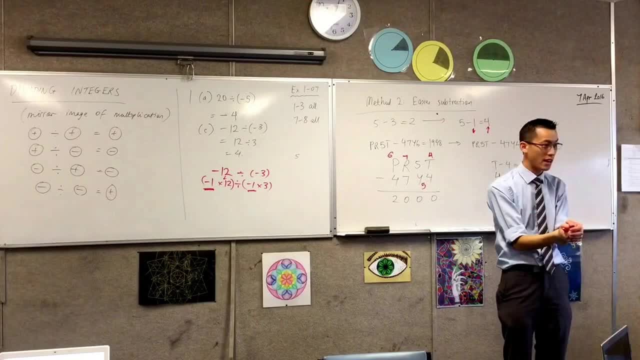 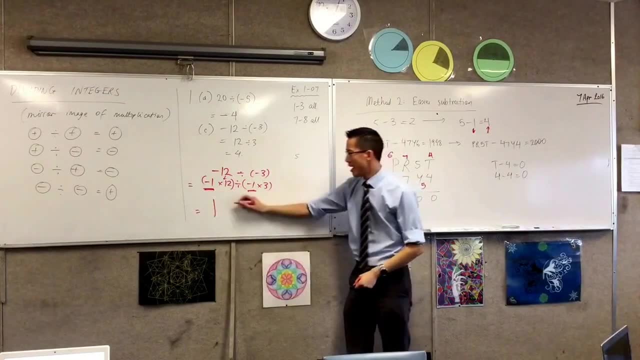 what happens when you divide a number by itself? You just get 1, right? So this is going to be the negative 1, and the negative 1 will just be 1 times 12 divided by 3, which, of course, you already told me is 4.. 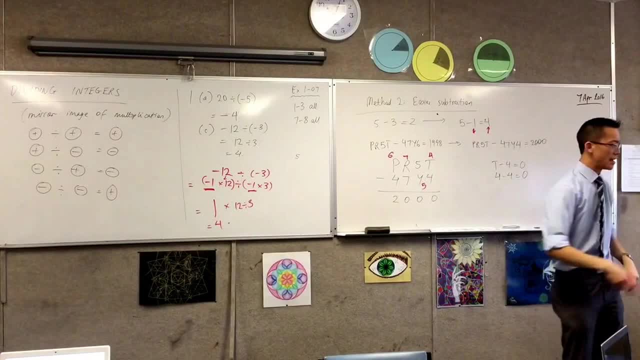 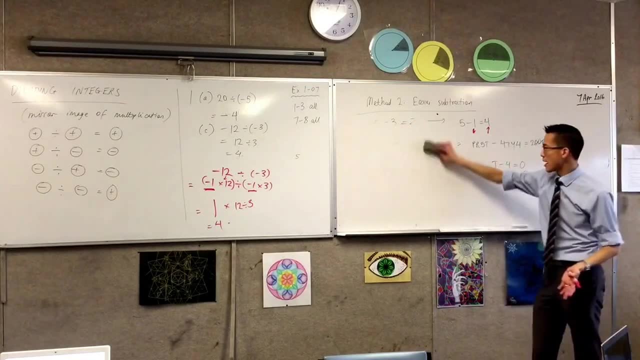 So these negatives are kind of cancelling out with each other. Now you remember I asked you to get your calculator out. This is about multiplying and dividing by positives and negatives, right? There is one special number that is neither positive nor negative. 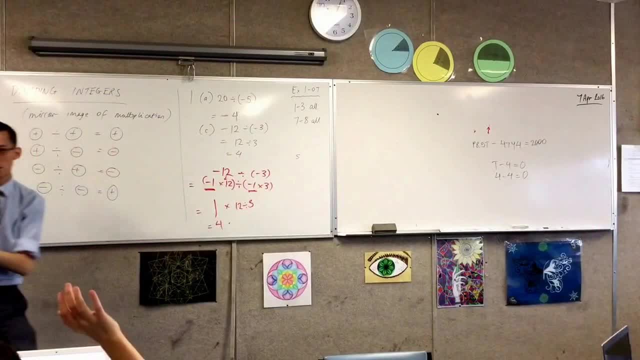 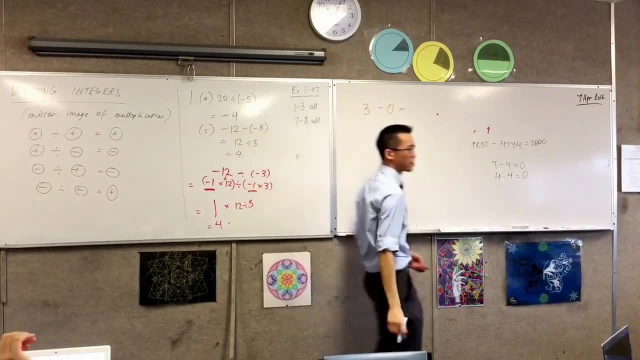 and that's 0, right? So question and don't shout it out. I want you to think about it first. What if I said 3 divided by 0? It's not in the exercise, and you'll see why in a second. okay, 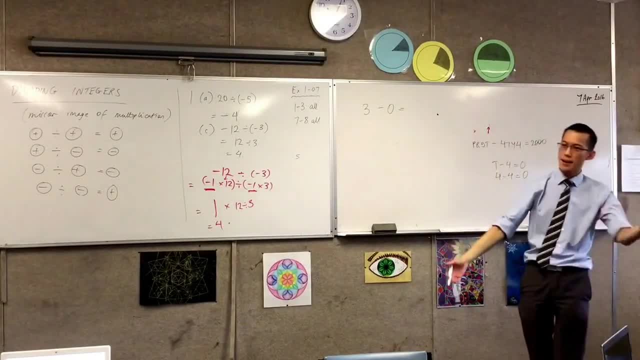 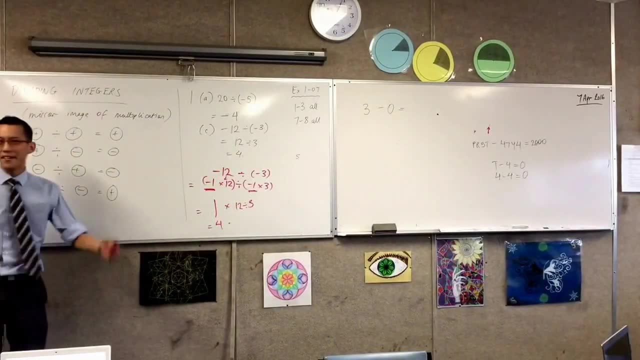 But it kind of begs the question: I can divide by positives, I can divide by negatives. What happens if I divide by something else? okay, Christian, what do you have as a suggestion? Nothing, Okay, Nothing. Anyone want to suggest something different to nothing? 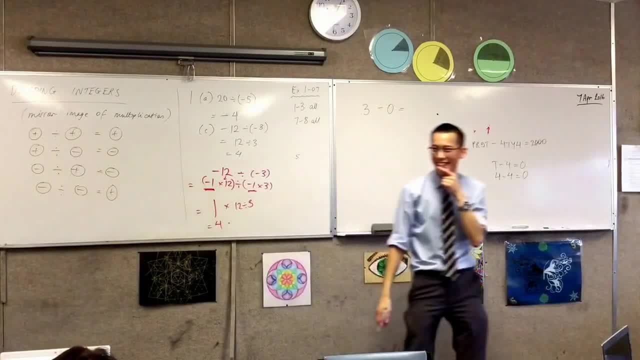 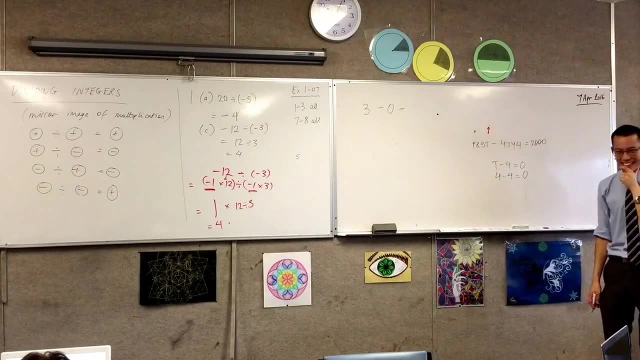 Nikhil, You get like everything, or you get an unspecified amount of a number because there's nothing you can divide it by, because, Never mind, Yeah, Okay, right, I get what you mean. Okay, So let's think about, for example, if I said 12 divided by 2.. 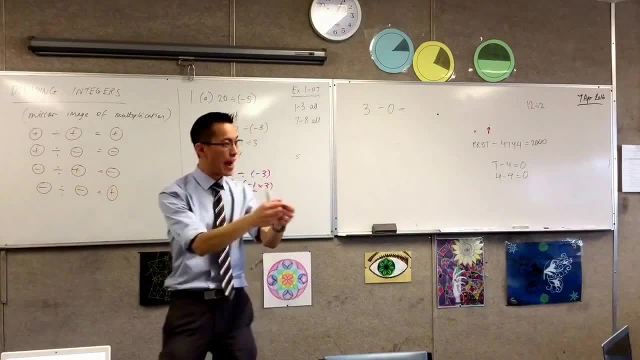 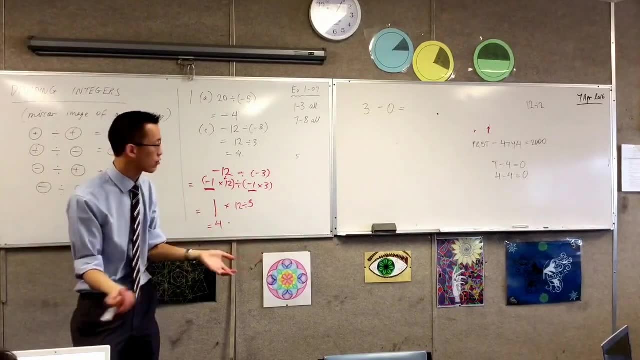 What that means is: okay, if I've got 12 objects and I divide them into 2 groups, okay, how much will be in each group? Does that make sense? And you guys know? okay, you'll have 6 in each group. 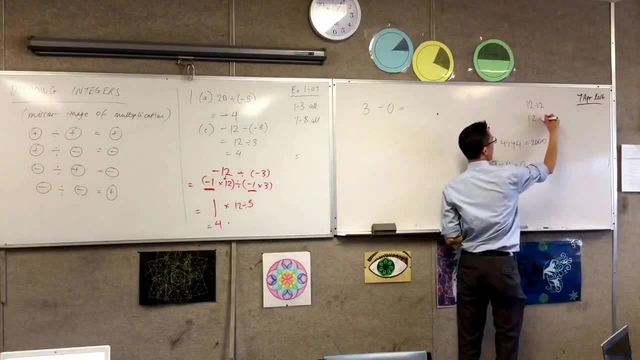 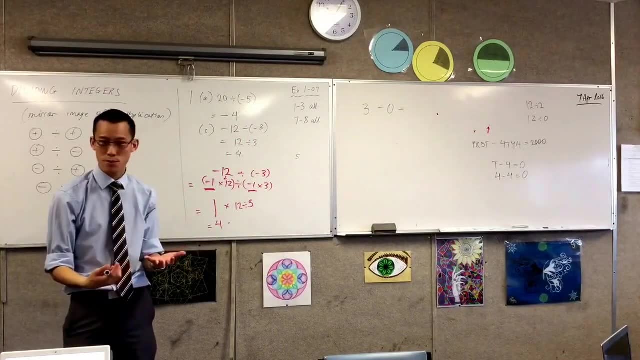 If I say: what about 12 divided by 0?? That doesn't make sense with that grouping idea, does it? If I have 12 things and I divide them into 0 groups, how big is each group? We don't really have an answer for that. 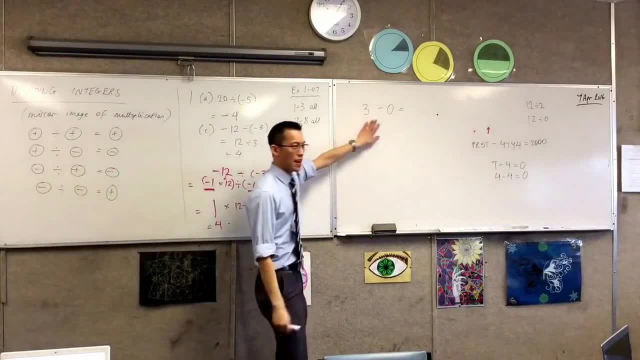 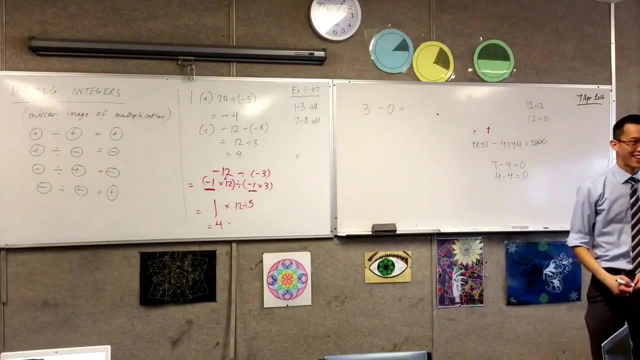 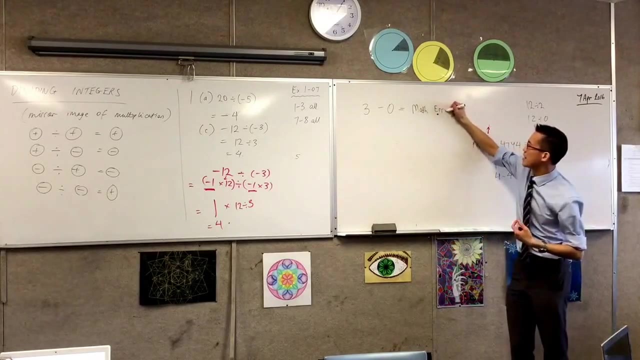 Now on your calculator. there, I'd like your original calculator and see what it tells you: 3 divided by 0 equals, And what does it say? This isn't a math problem. You've done something funny with yours, My calculator. usually it says I'm not happy, and it flips the table and it goes home. 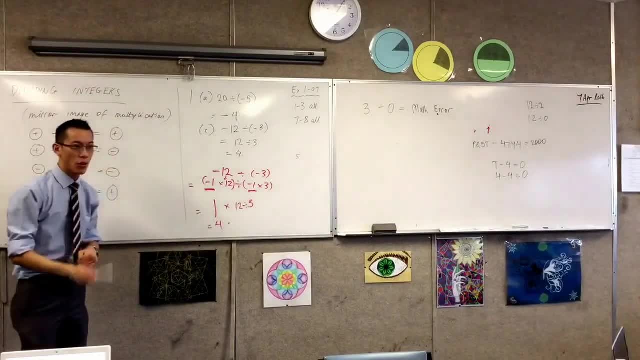 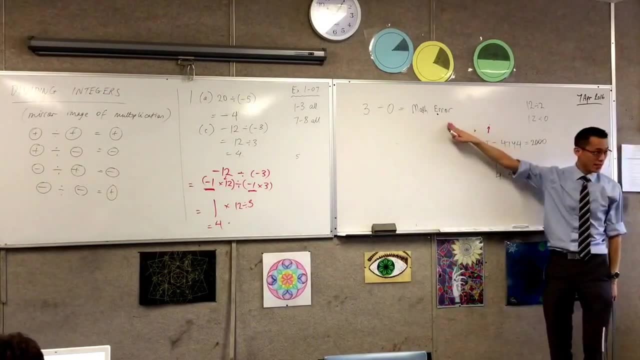 Okay, Now what's going on here? Let me tell you what's going on. Yes, On my laptop it says: cannot divide by 0. Yeah, that's right, But it doesn't give us an answer, nor does this as to why. 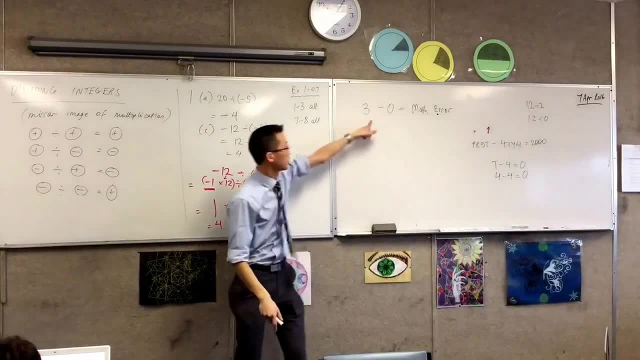 Let me help you understand What's the question. Oh, shh, That's the question. Oh, okay, Okay, Let me show you what's going on. Right, 12 divided by 2.. Can you tell me what 12 divided by 2 was again? 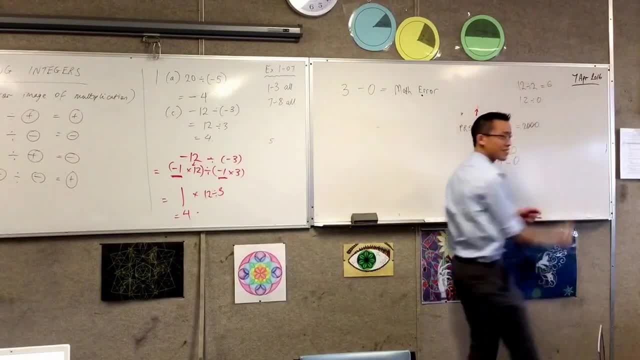 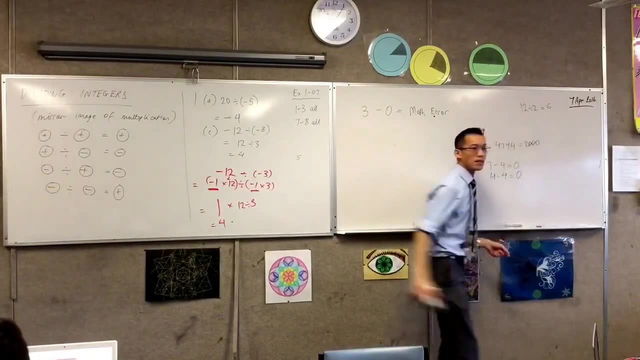 It's 6.. Okay Now, just like we did at the start of the lesson, can you turn that division statement? can you turn it into a multiplication statement with the same numbers, 2 times 6.. 2 times 6.. 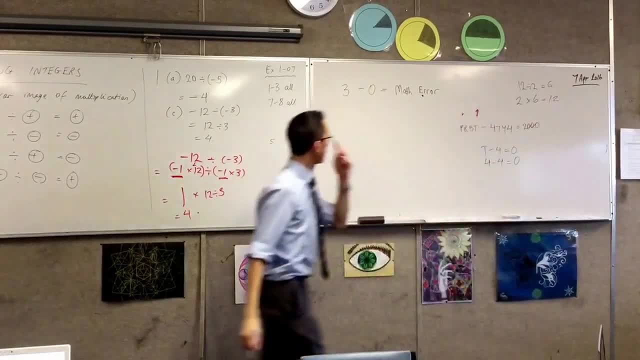 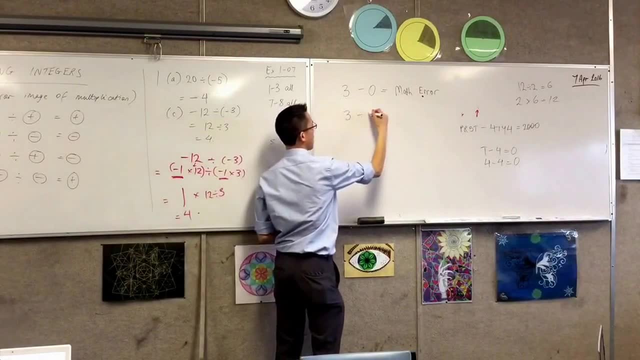 Good, That equals 12.. Okay, Now let's just suppose that 3 divided by 0 was an actual number. Okay, 3 divided by 0 was something. I'm going to make it a star. Okay, Because I like stars. 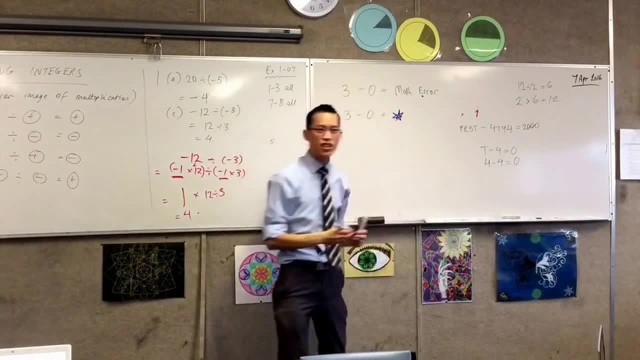 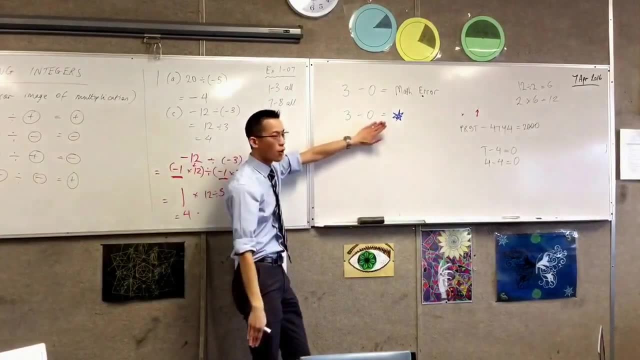 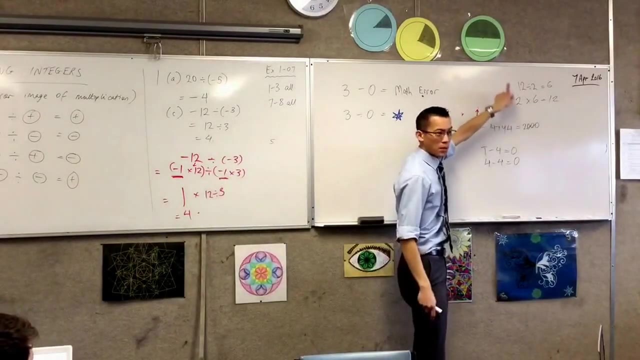 I like stars. Okay, Now just imagine this was a real number. Okay, What would that mean? What multiplication statement would go with this that uses all the same numbers? Can someone tell me What multiplication statement would be the opposite of this division statement? 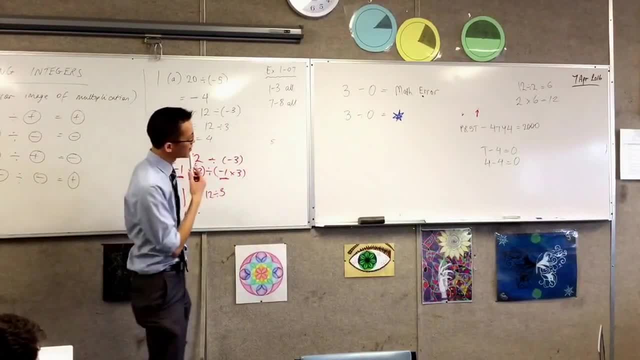 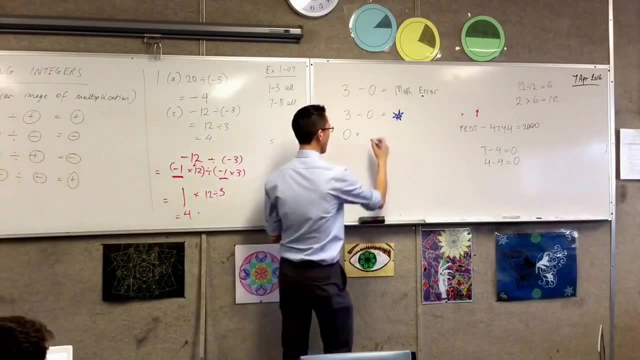 Have a look. Look at it carefully: 0 times, 0 times star. I think it's going to be 0 times Star. My blue star, Which is going to be 0 times star, My blue star, Which is going to be 0.. 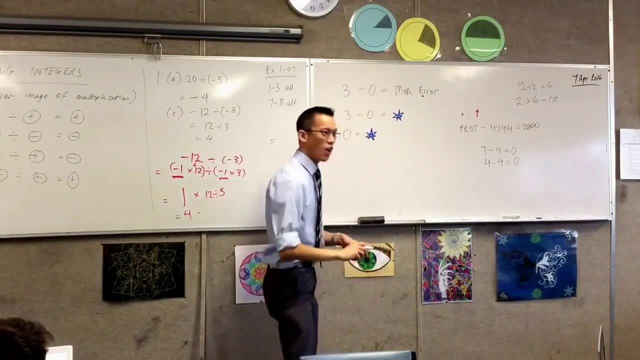 Is going to be equal to 0.. Well, now hold on a second. According to this, it should be 3.. But something's gone wrong. Something's gone terribly terribly wrong. Right 0 times anything Equals 0.. 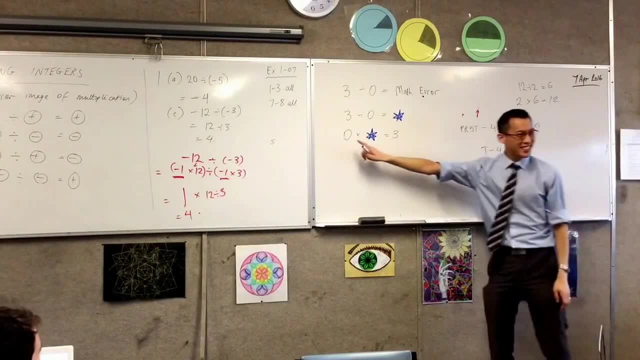 I don't care if it's 12 or 6 or a star or Nikhil. 0 times anything should be 0.. Is this equal to 0?? Mine's true. Mine's true. I'll have to have a look at what you've done here. 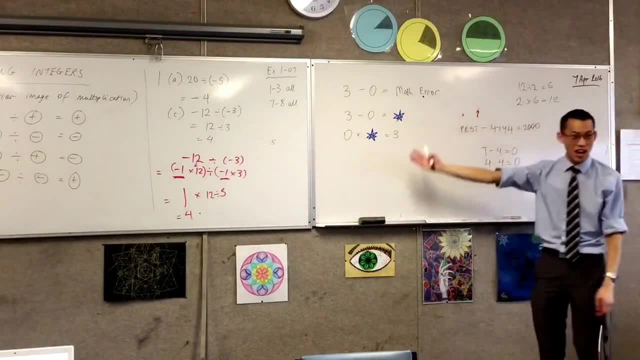 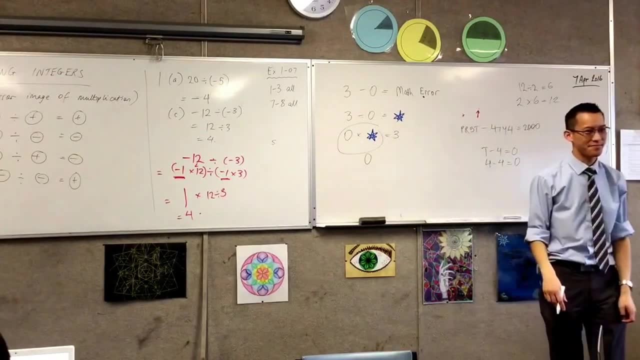 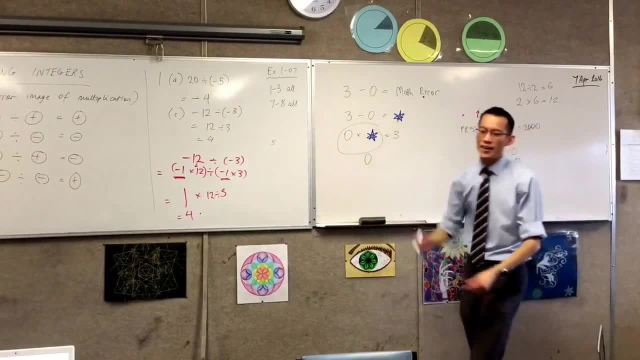 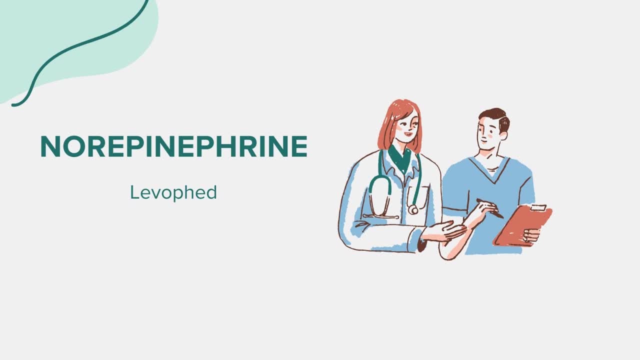 Welcome everyone. Today we're exploring a critical medication in emergency medicine and intensive care units, norepinephrine, also known by its brand name LevoFed. This session is designed for educational purposes only For personal health queries or concerns.